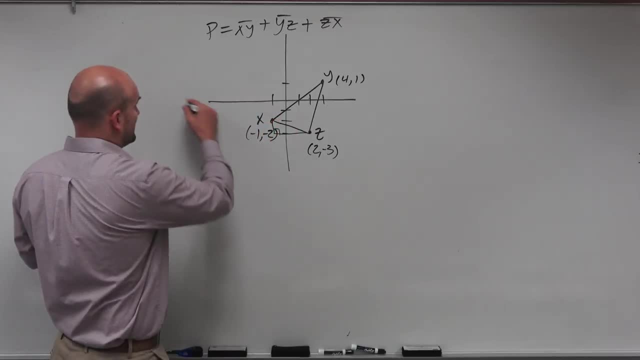 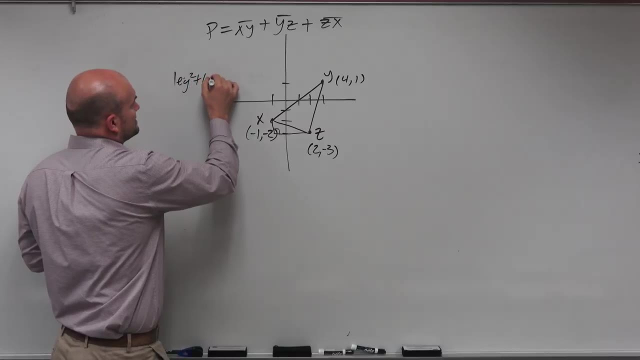 leg squared plus leg squared equals my hypotenuse squared. So again, if you recall, what we did was if we have leg squared plus leg squared equals the hypotenuse squared. well, if I need to find the hypotenuse, which is the distance, then that's the distance. 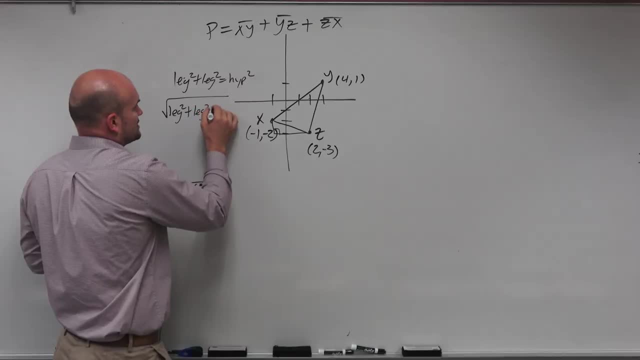 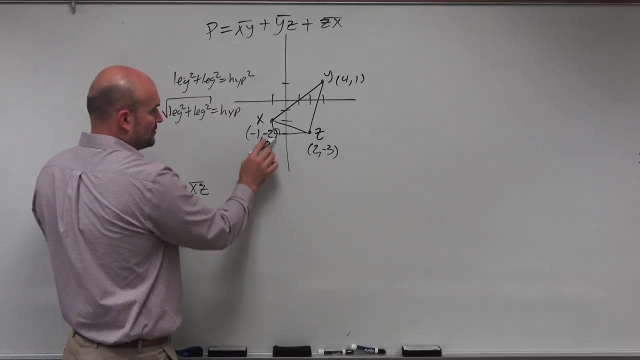 That's just going to be the square root of leg squared. plus leg squared equals hypotenuse, which again represents the distance. So let's go and do that. So this length we can just count. since it's on a coordinate grid, We can say: from there to there And again the 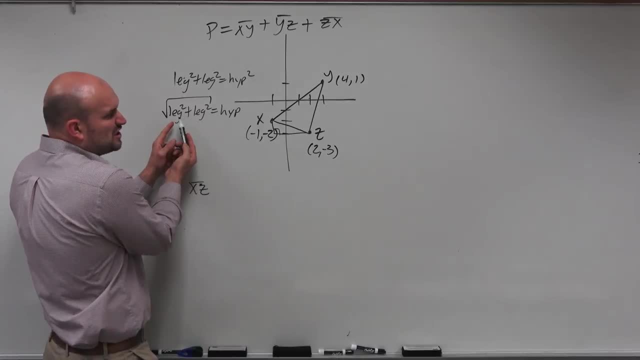 issue here is: it doesn't really matter, But since your leg is being squared, we're just looking for the absolute value of distance. You're just counting. You could say that's going to be a distance of 1.. You go from negative 1 to I'm sorry. 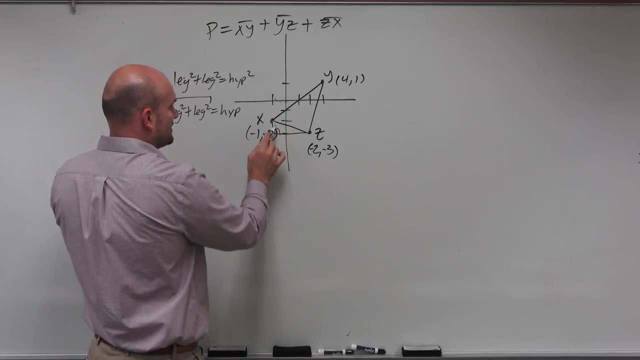 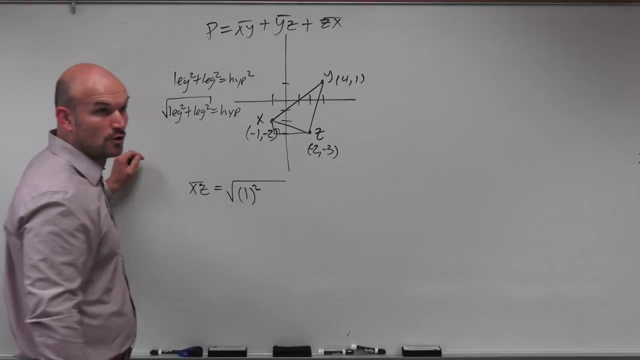 0.. 0.. 0.. Negative 1 to negative 2.. So negative 2 to negative 3, yeah, So you're in a distance of 1.. And it doesn't matter if you use positive or negative, Because it's going to be squared, so it's going to be positive. 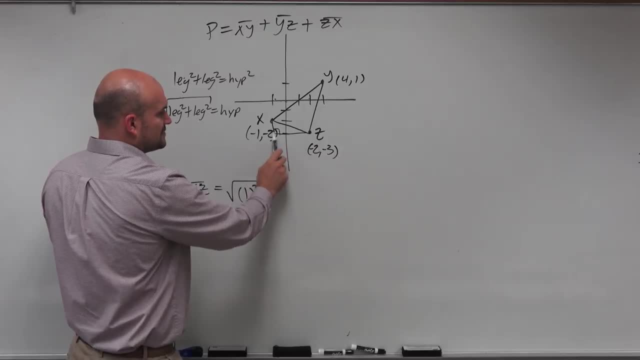 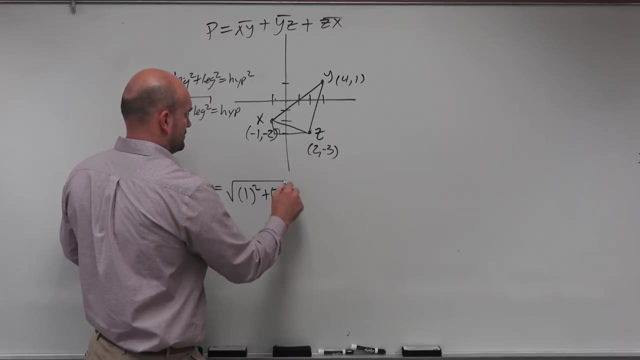 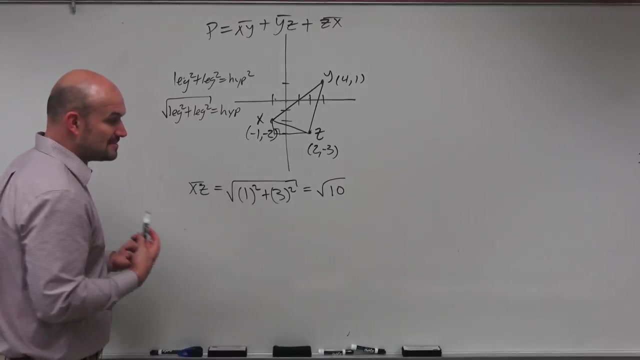 Plus, you have to go from negative 1 to positive 2.. I did have that right: Negative 1 to positive 2, you can just count 1, 2, 3. Plus 3.. So that's going to equal the square root of 10.. So sometimes it's easy to count and sometimes 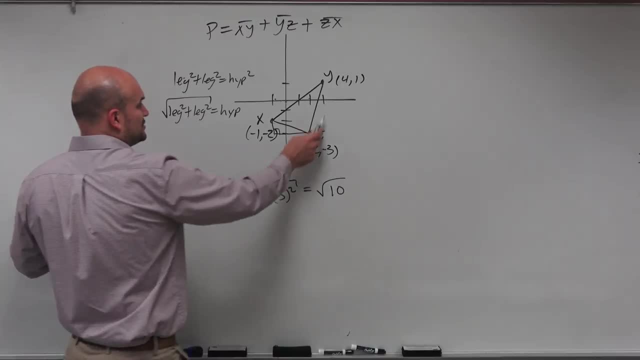 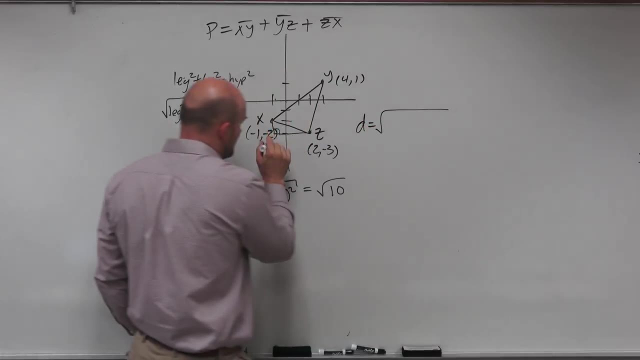 like you can quickly count it. Other times it just might be easier to do the distance formula. And if you remember the distance formula, we're doing the same thing. but rather than counting, you can also just find the difference between the horizontal and the vertical lengths. 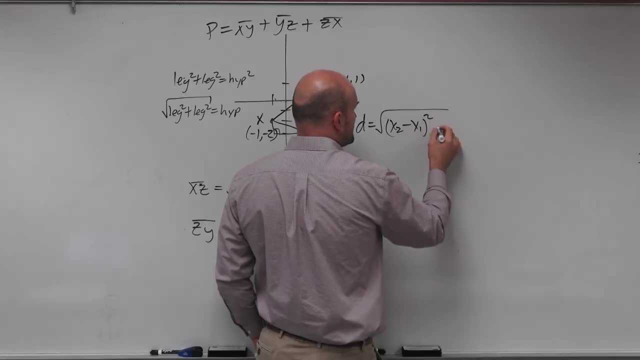 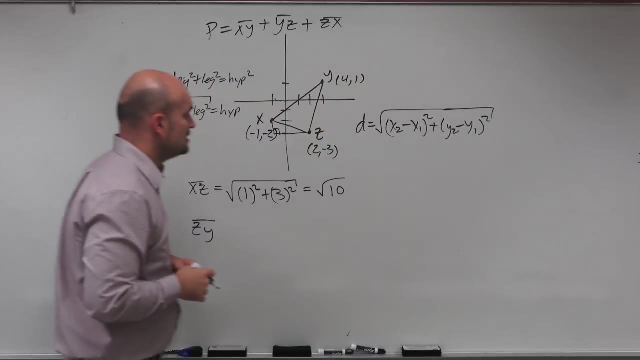 Because when you find the distance between those lengths, that gives you how far something is. So that would be y2 minus y1, cosine squared. So now, here's the important thing: Which one is your x2, y2?? Which one is your y1, x1?? 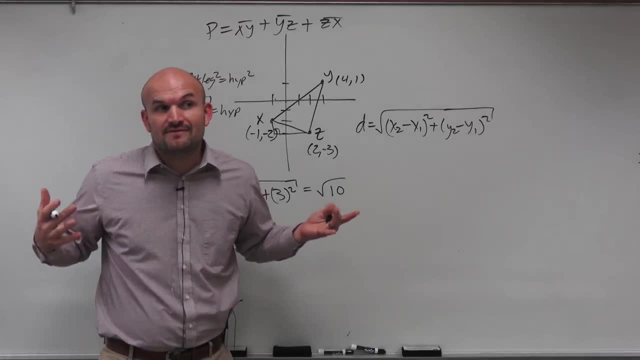 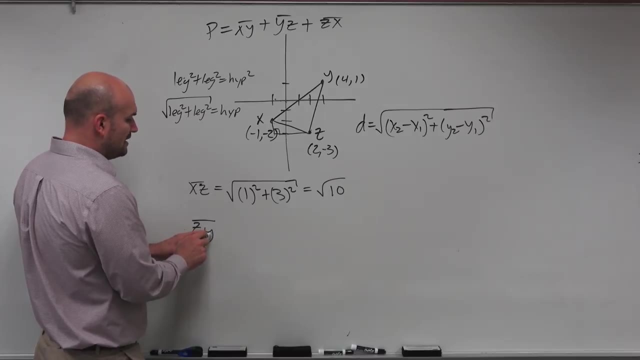 It doesn't matter again, because it's either going to give you a positive or a negative value, and the value gets squared. So what I like to do is I like to always have z be first and then y. So this is going to be my x1, y1,. 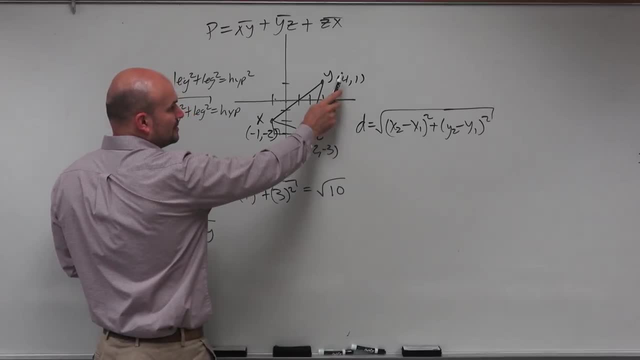 and this would be my y2, x2.. So again, you're subtracting your. so if you're going to go from z to x, you subtract y or z to y. if you're going to go from z to y, 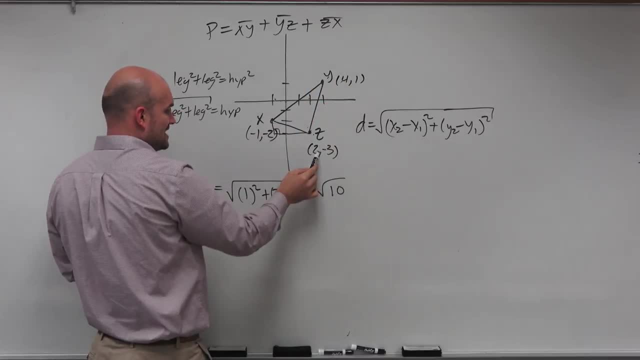 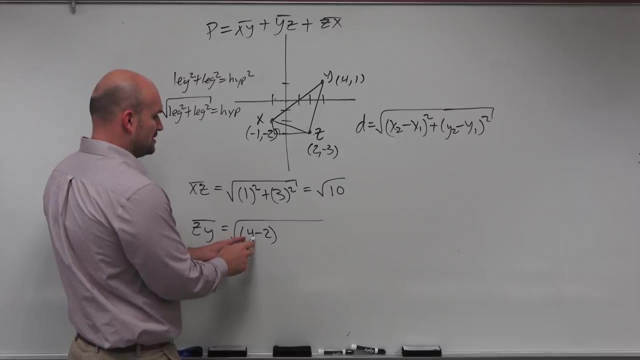 you subtract here from there, So again it's x2 minus x1.. So I'll just write it out For this first one, and then I will do the same thing, but I'll do it quicker. So 4 minus 2, quantity squared plus 1 minus a negative 3.. 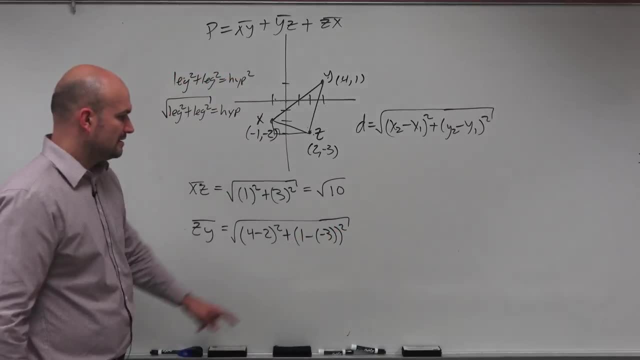 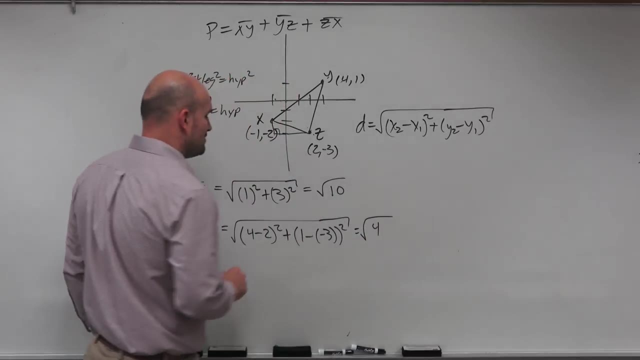 Notice my use of parentheses. It's minus a negative 3.. So 4 minus 2 is 2.. 2 squared is 4. And 1 minus a negative 3 is 4.. 4 squared is going to be 16.. 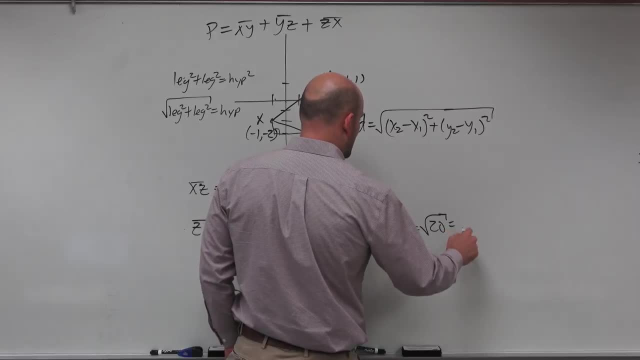 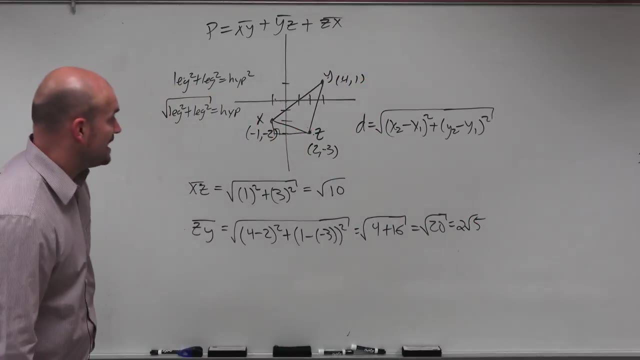 And therefore that's going to equal the square root of 20, which you could go ahead and simplify to give you. We could go ahead and further simplify that to give you a 2 radical 5.. And then the last one, let's just do x, x. 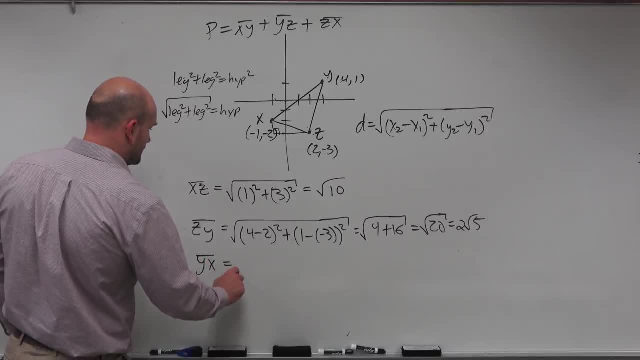 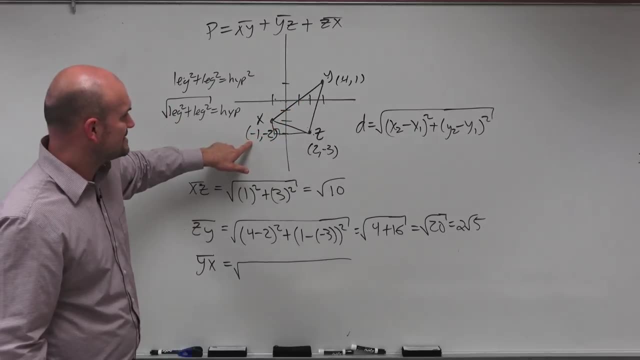 No, let's do y, x. So if I want to find the distance here again, I'm going to do the same thing. But I'm just going to kind of do this in my head now: 4 minus a negative 1 is going to be 5.. 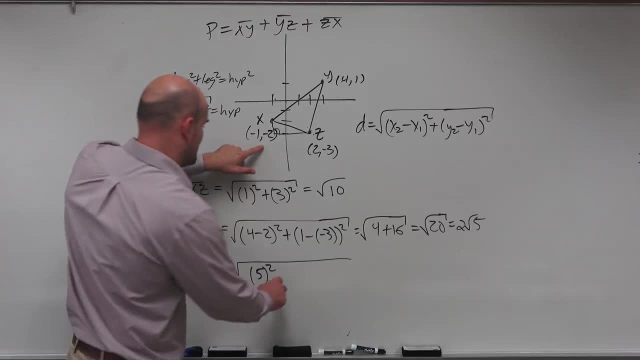 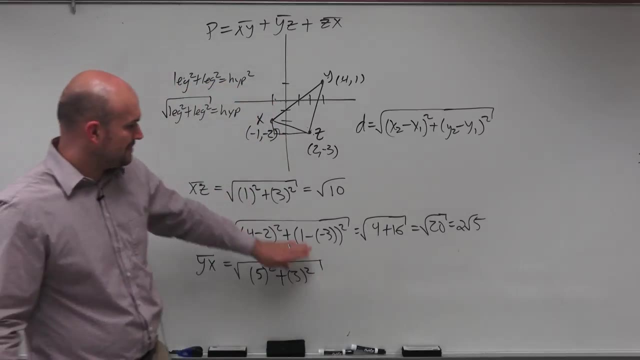 And then here I have 1 minus a negative 2, which is going to be 3.. So the faster you get at this, the easier it's going to become. But again, you've got to be careful with these negatives. 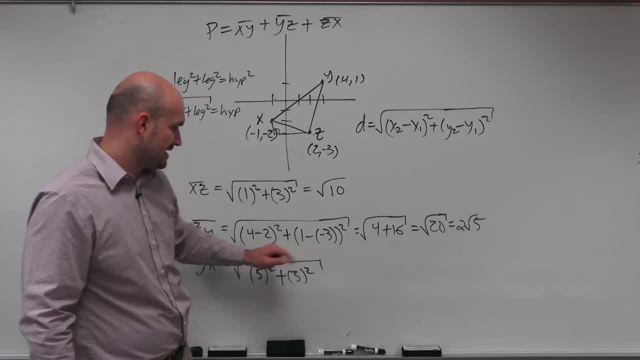 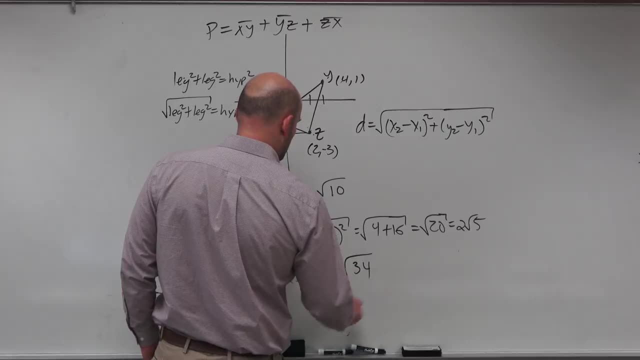 That's why this is helpful to write it out, so you don't make those mistakes with the negatives. And therefore you have: 5 squared is 25 plus 3 squared is 9.. So that's going to equal the square root of 34.. 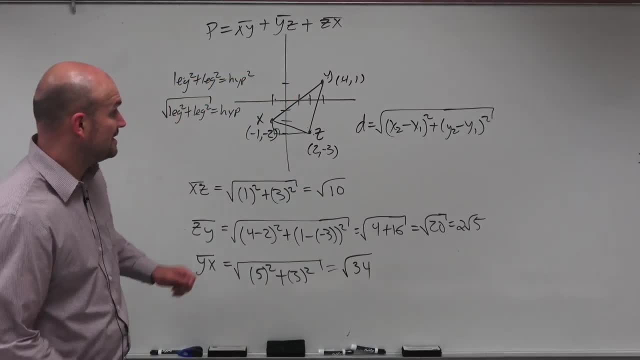 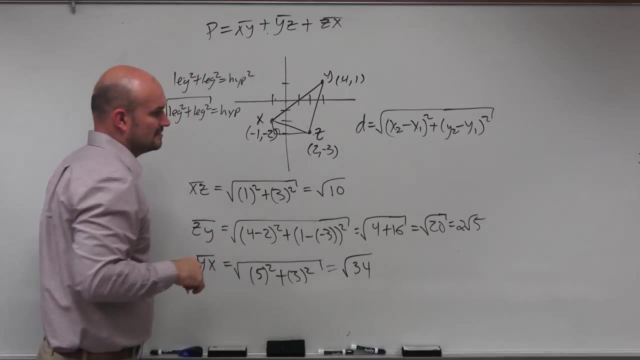 And that one we cannot simplify, So we'll just leave it as that. And then we are not done, though I almost got it. Remember, guys, we're finding the perimeter. The perimeter is the sum of all the sides. 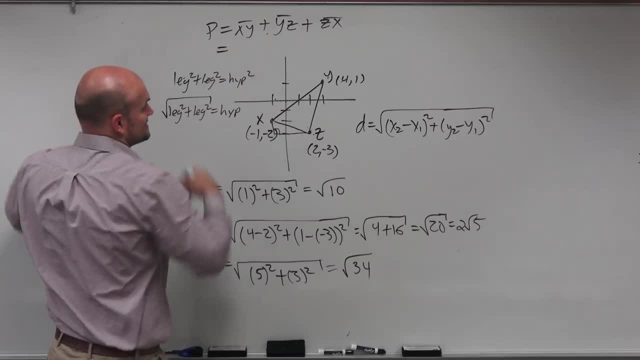 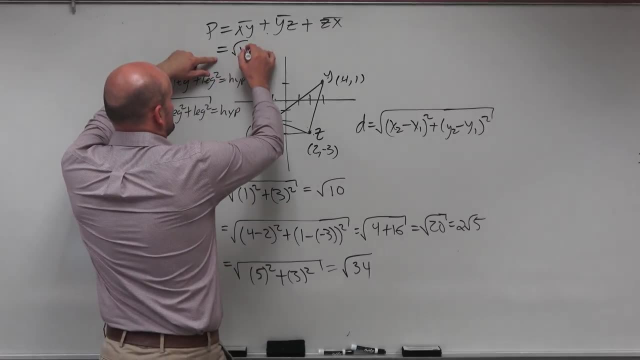 OK. OK, So the perimeter- and I'm going to leave it as an expression because I don't have a calculator with me. so that's OK. Hopefully you guys can check my work. We have xy, which is square root of 10, plus yz or zy. 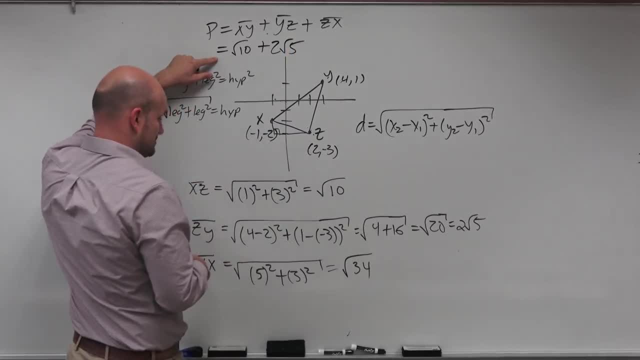 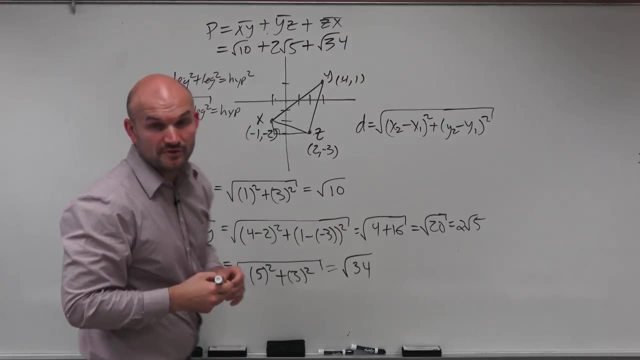 doesn't matter. is 2 square root of 5.. Or you could just do square root of 20.. And plus yx is going to be square root of 34.. OK, So there you go. ladies and gentlemen, That is how you find the perimeter of a triangle using 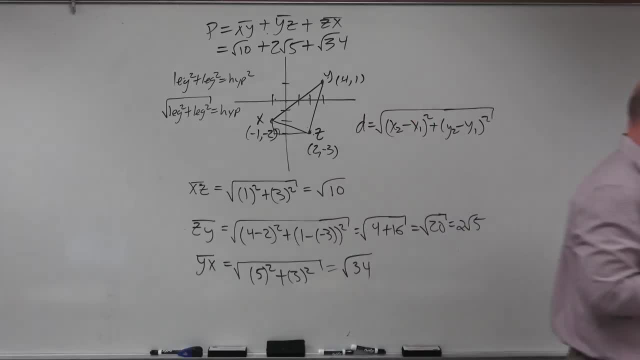 the distance formula and Pythagorean theorem. Cheers.